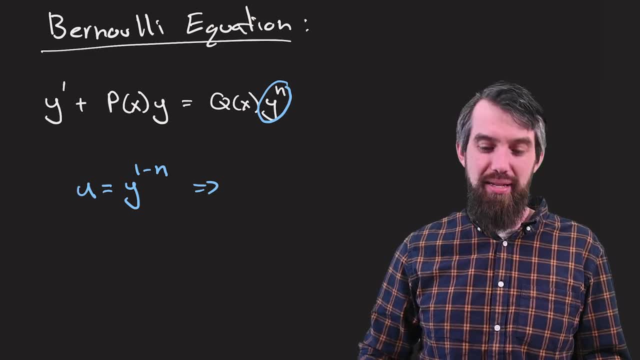 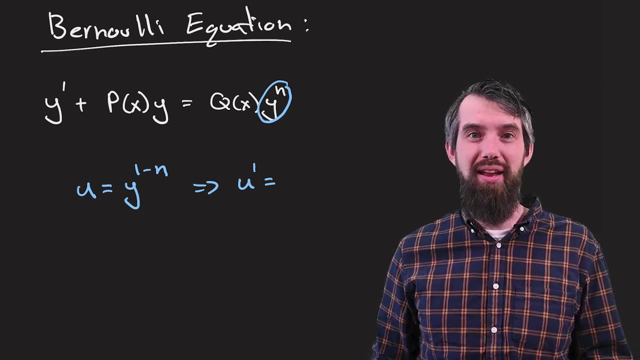 able to do. u and y are both functions of x. I want to make some claim about what u prime is going to be. Well, indeed, this is going to be the derivative of y to the 1 minus n, and that I can do by chain rule. So this: 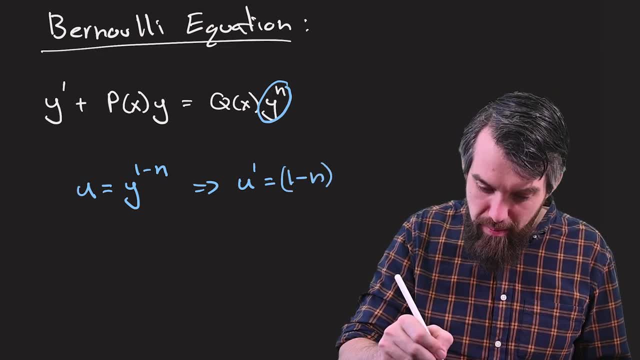 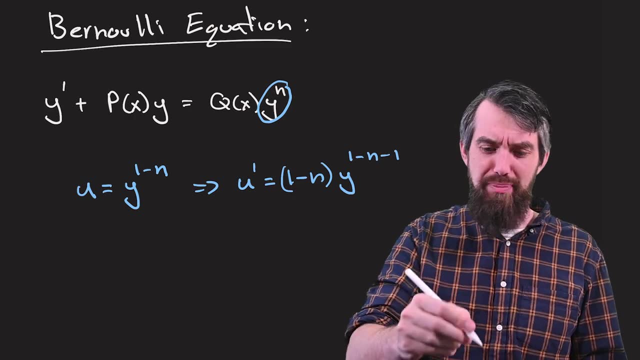 is going to be 1 minus n is going to come out the front, and then this is multiplied by y to the 1 minus n, but 1 less than that when you take the derivative. so minus 1.. And perhaps instead of writing 1 minus n, minus 1, I'll just write minus n And then multiplied. 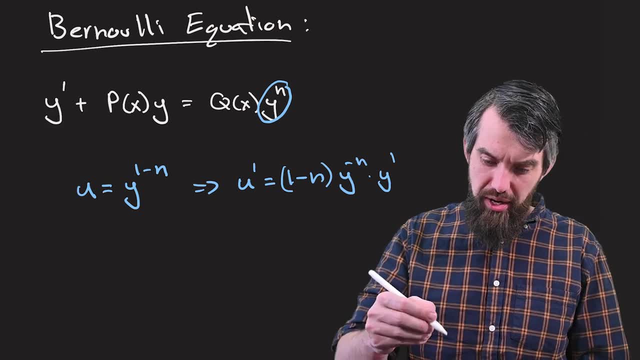 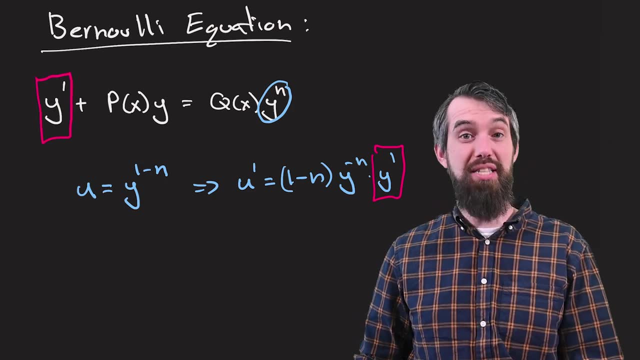 by y prime. So what that will mean is that I have this y prime appearing in my u prime formula, but then I also can connect this to the original equation because I have a y prime there as well. So what I'm actually going to notice- and I've already circled it once, but I'll 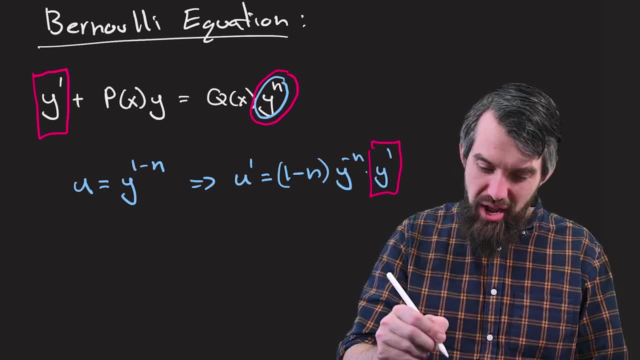 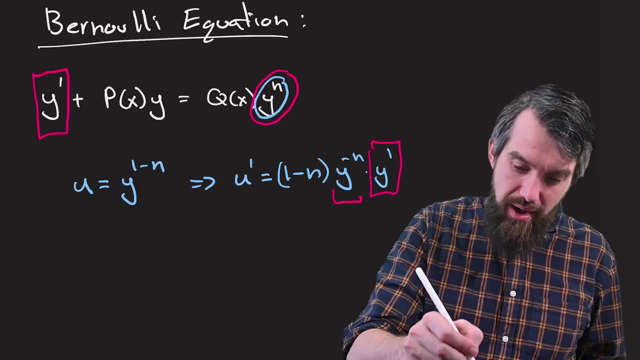 circle a second time. I've got that y to the n in the original equation and I also have a y to the n, except it's on the bottom. So why don't we just align this? I'll just divide out the equation by y to the n, So that's going to give me y to the minus n times y, prime plus p of x times y to the minus n. 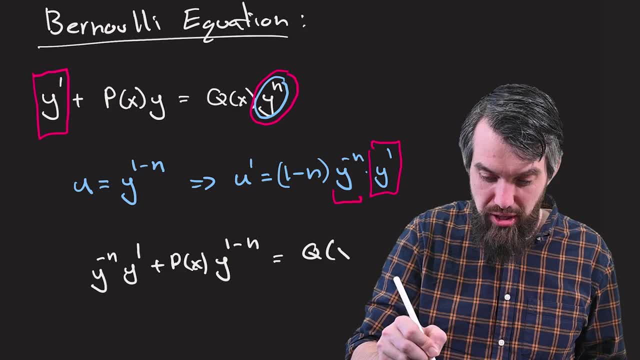 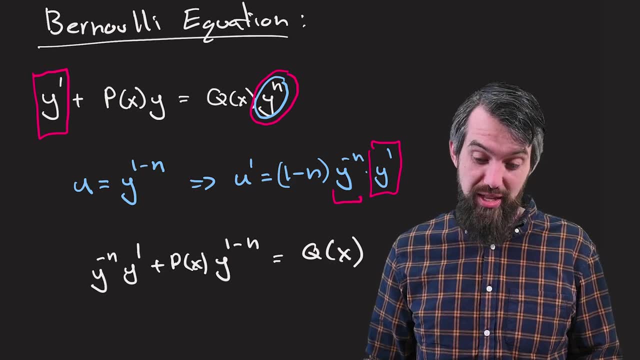 y to the 1 minus n is equal to q of x. So that's our differential equation, where I just divide it out by y to the power of n. And then I can look at the left expression, And this is pretty darn close to my expression for u prime. 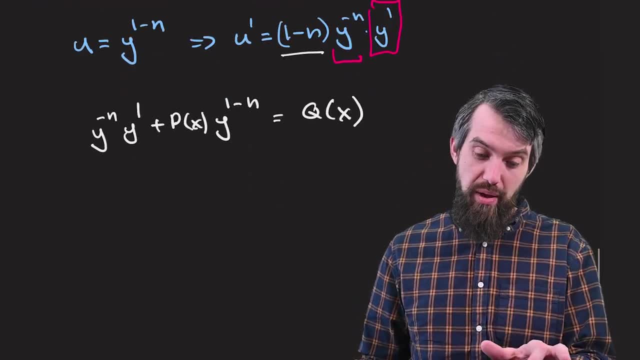 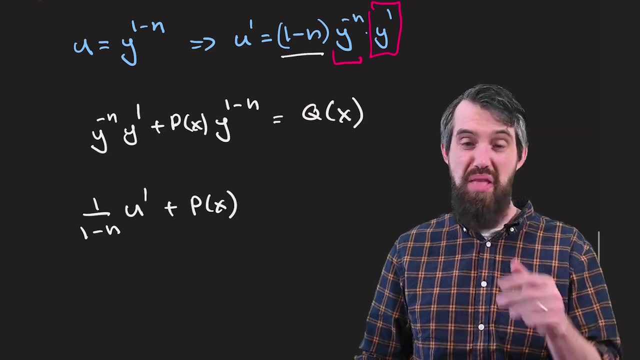 The only thing that's missing is this: 1 minus n. So if I plug this in, this is going to give me 1 over 1 minus n times u prime. Then I'm going to have a p of x And then y to the 1 minus n. 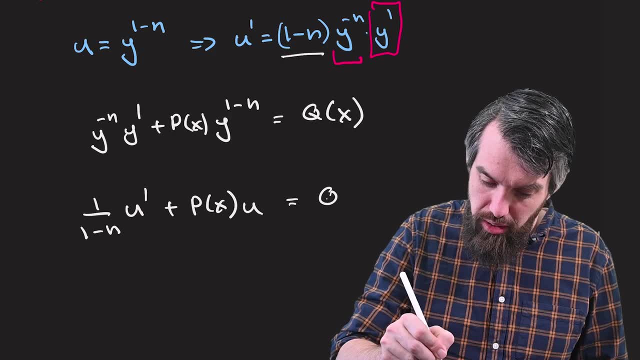 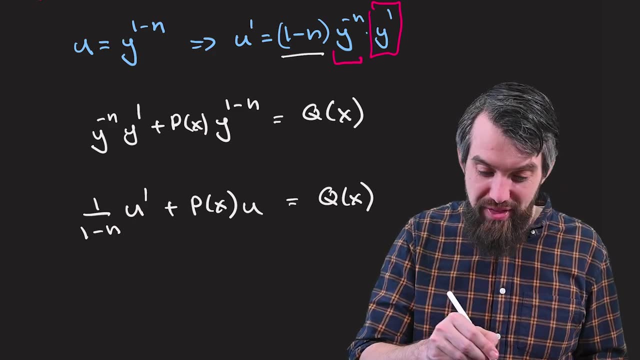 Well, that was exactly u, So I have a u here, And then just equal to q of x. All right, So I've made a change. And look what's happened In this change of variables, the equation that I have. this one is now a linear first order equation. 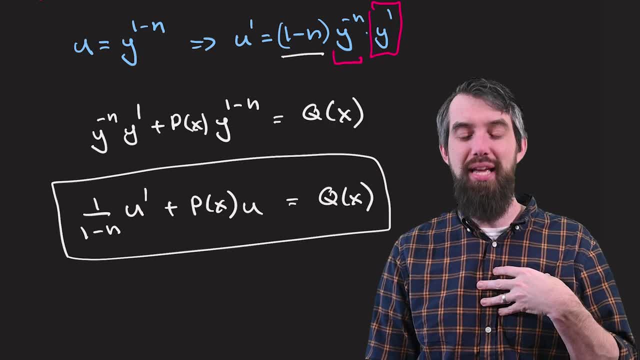 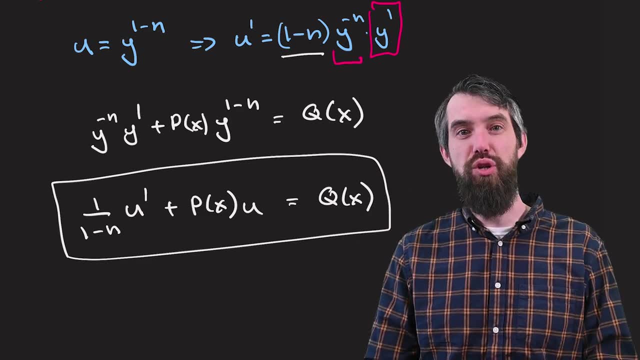 It's got a u prime with a coefficient of 1 over 1 minus n. It's got a u with a coefficient of p of x And it's got a 1 with a coefficient of q of x. This is a first order linear differential equation. 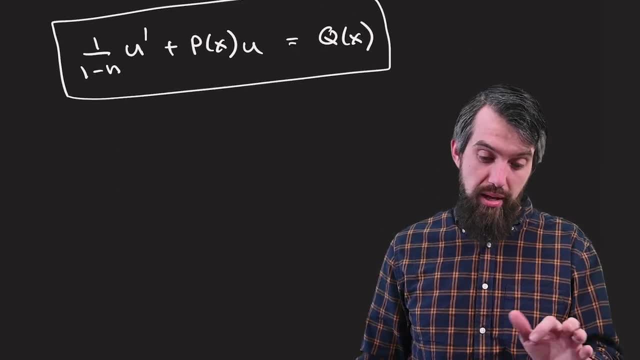 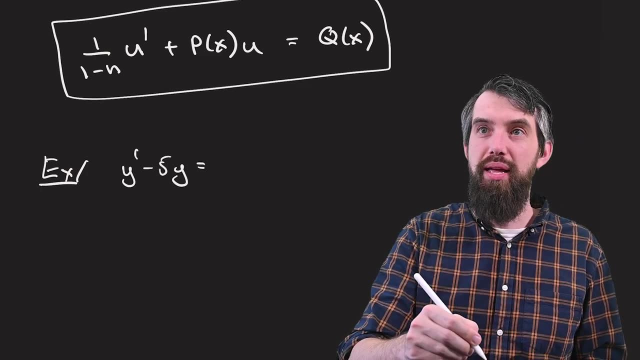 OK, So let's see how this works out in a concrete example. So I'm going to come and do as an example the following: y prime minus 5.. Times y is equal to minus 5 halfs xy cubed. 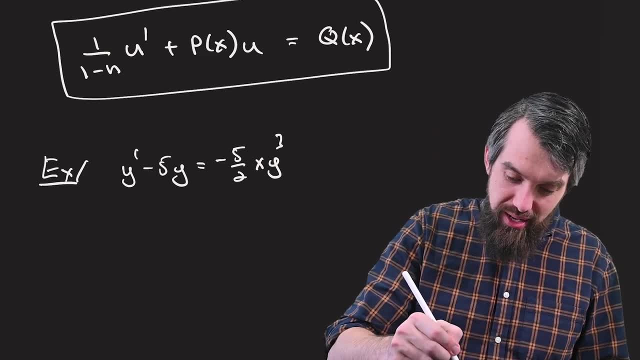 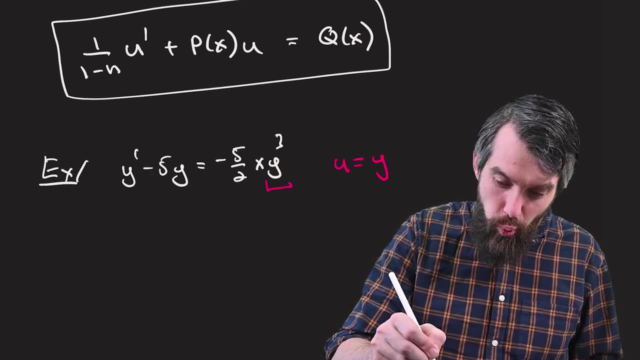 That's my messy expression, And so what I observe here is that this is a Bernoulli equation with y cubed, And so what I want to do for my change of variables is: u is y to the minus 2.. I then continue the method, which first involved taking a derivative. 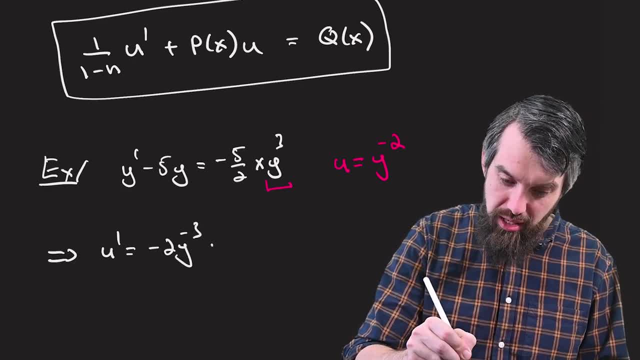 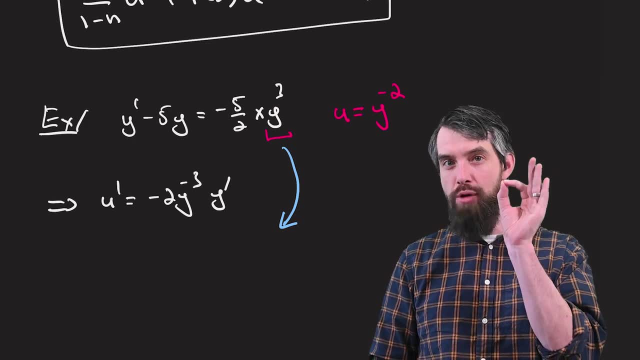 So this is minus 2y to the minus 3 times y prime. I'm going to take the original equation And I'm going to now rewrite it, dividing out by y cubed in my head. So when I divide out by my y cubed in my head, I notice that, first of all, 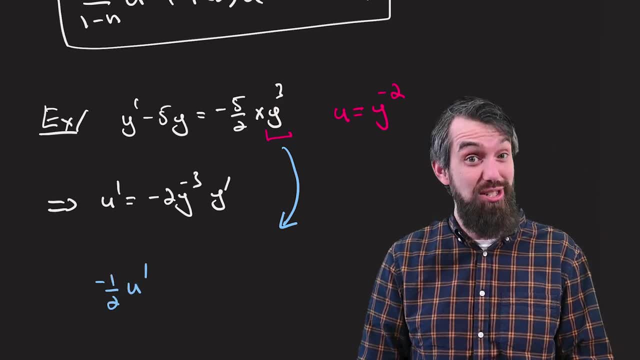 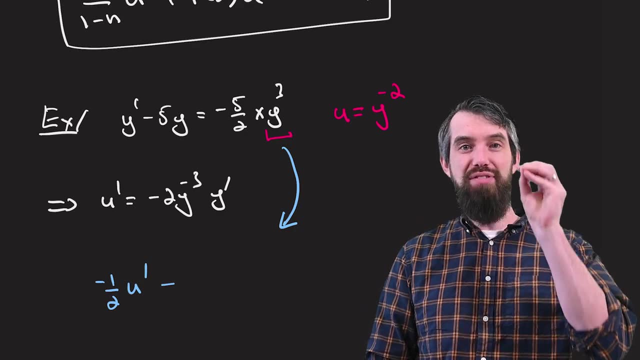 I'm going to have a negative 1, half times a? u prime. That's because there was a minus 2. And I'm changing it over to the other side. So minus 1 half, And then I'm going to have a minus 5 times y divided by y cubed is y to the minus 2.. 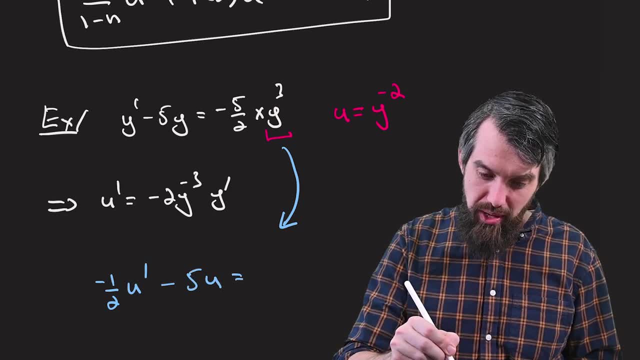 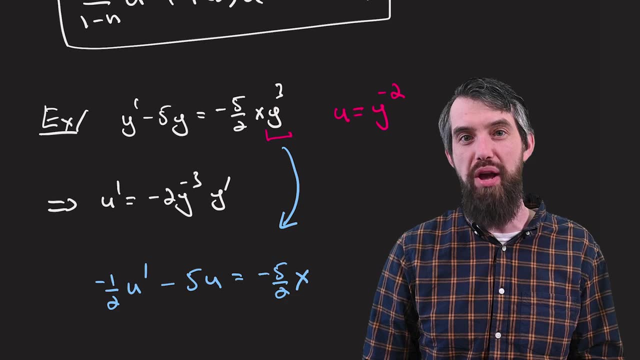 So there's minus 5 times u, And then this is going to be equal to minus 5 halfs times x, And now there's no longer a negative. It's going to be 1 over y cubed, divided the entire equation by y cubed. 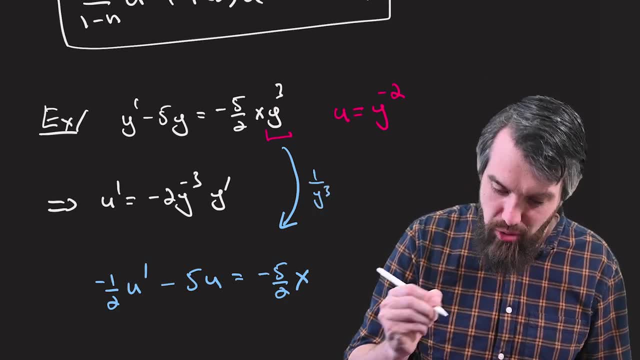 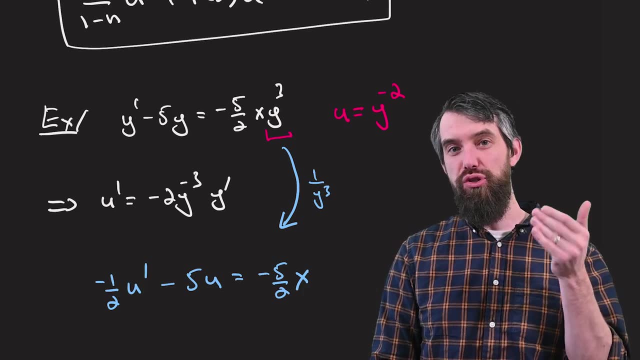 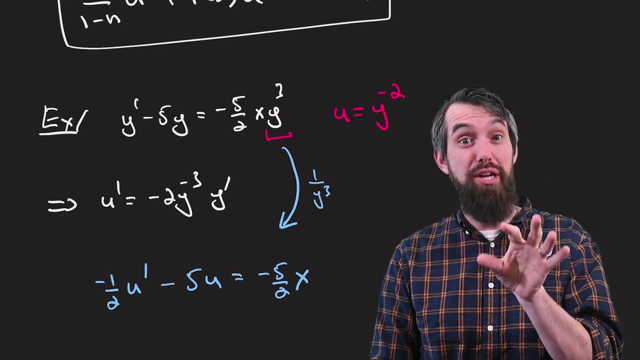 Maybe I'll put that in explicitly- that I was doing a 1 over y cubed and changing to u's when I did this, And what I have now is an example of a first-order linear equation, as we expected. So now I'd actually encourage you to pause the video and see whether you can solve this first-order linear equation yourself and see whether you get the same answer I do. 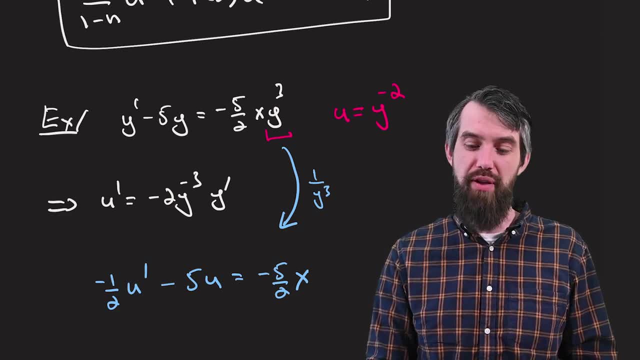 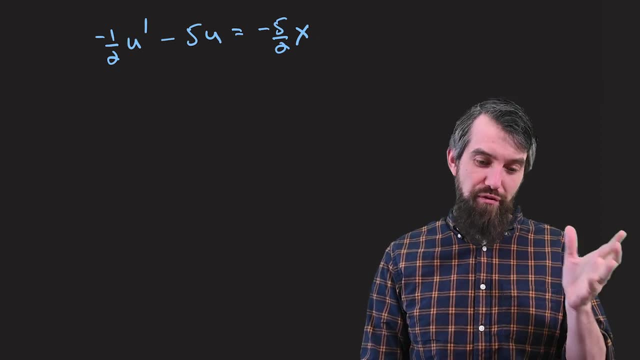 And if you just want to enjoy the show, well, here's my attempt at the method of integrating factors. So when I look at this equation, the first thing I note is it is linear, u prime with the coefficient function of minus 1 half. 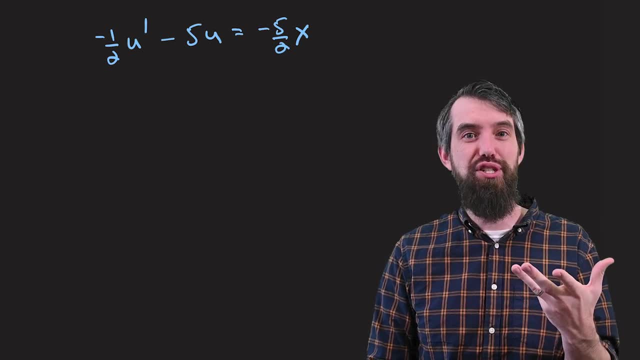 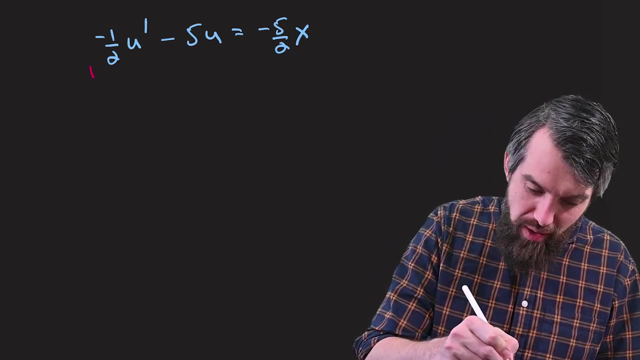 u with the coefficient function of minus 5.. And 1 with the coefficient function of this minus 5 halfs times x. It's not actually yet in standard form, So that's a little trick. We've got this minus 1 half here. 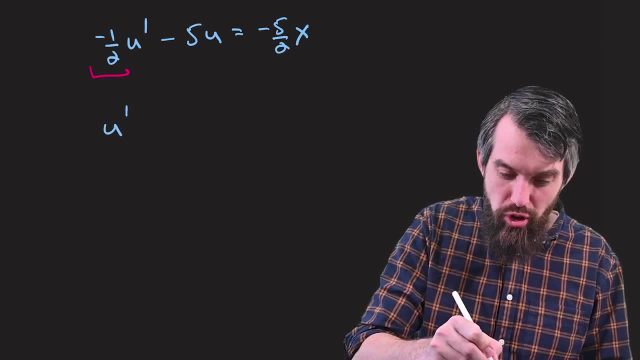 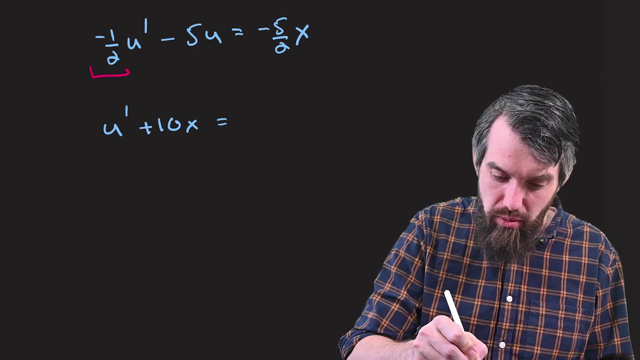 So if I want to convert it to standard form, which just has a u prime out the front, then I'm going to multiply everything by minus 2.. So that's going to give me plus 10x, And then that's going to be equal to 5 times x. 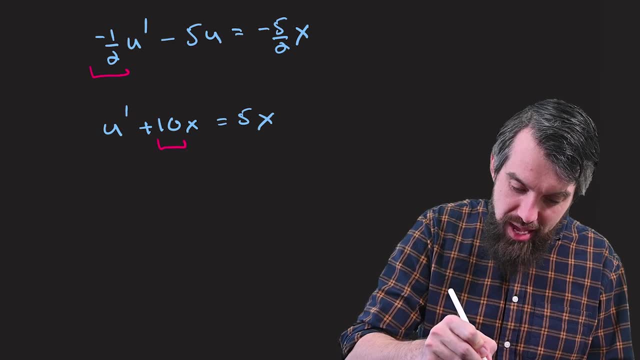 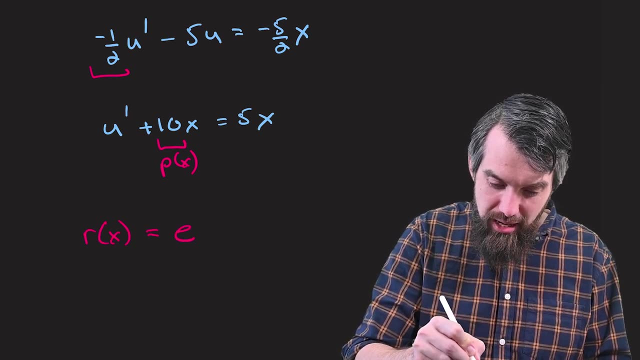 That makes it a little bit cleaner. And then I'm going to go and look at this: That is my p of x And I use my p of x to get my integrating factor. Integrating factor is r of x, is e to the power of the integral of p of x, dx. 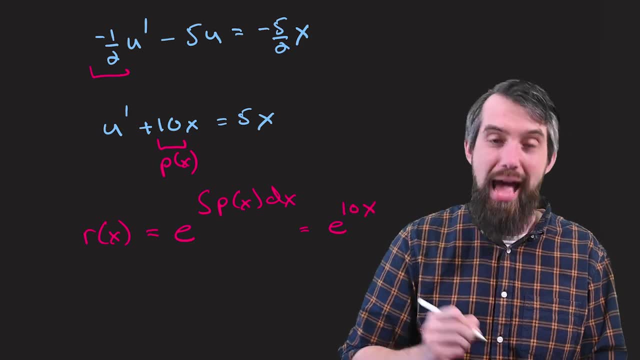 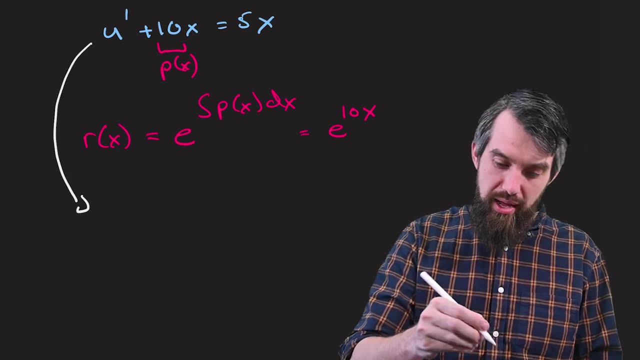 which in this case is just going to be e, to the power of 10x, And again the plus c. I'll just arbitrarily set it to be 0.. So then, what does an integrating factor do? It multiplies all the terms. 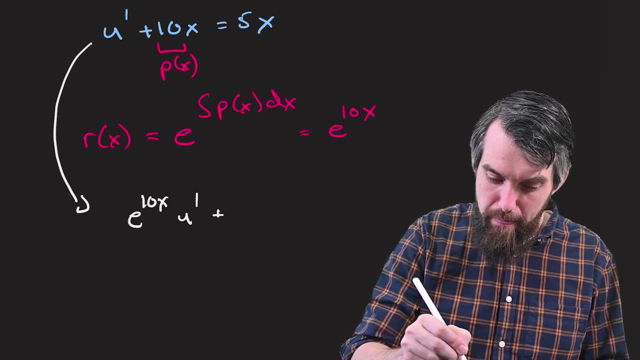 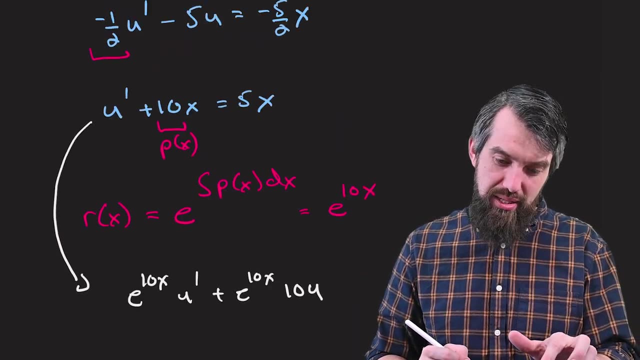 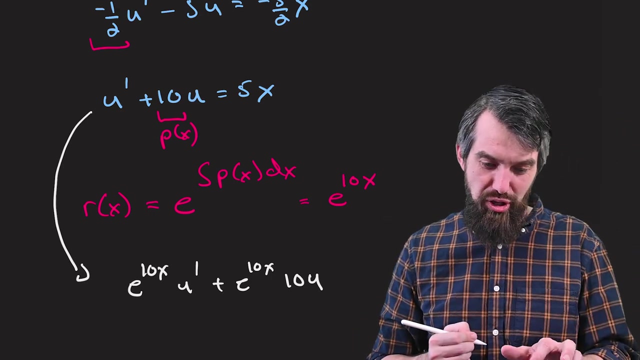 And so I have an e to the 10x times u. prime An e to the 10x times 10 times u. I see now that I had made a slight typo. I wrote plus 10x earlier. I meant plus 10 times u, so I've corrected it down below. 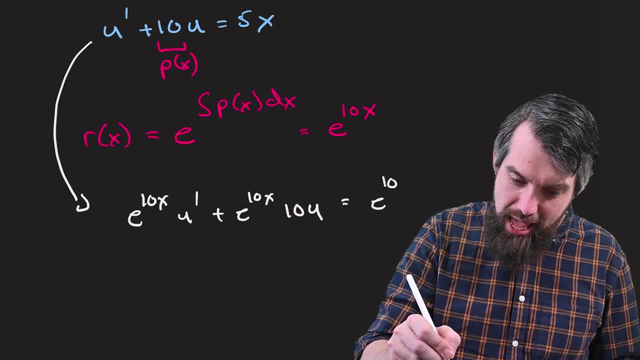 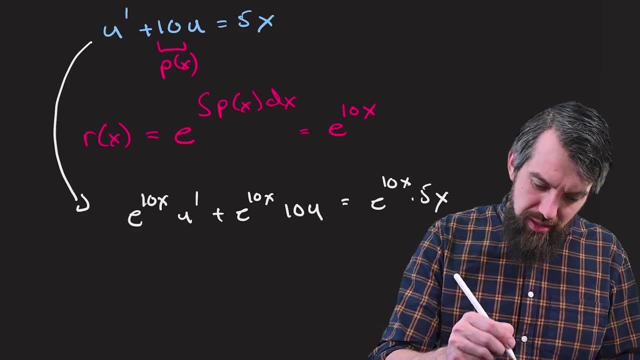 All right, let's carry on. Is equal to e to the 10x times 5x, And the one on the right-hand side is supposed to be an x. And then we use the standard trick that we can do every time when we're doing the method of integrating factors, which is: 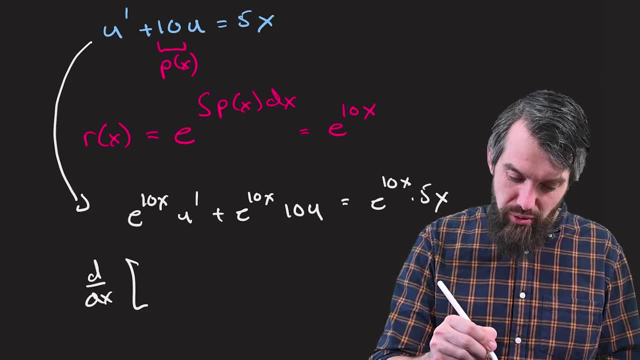 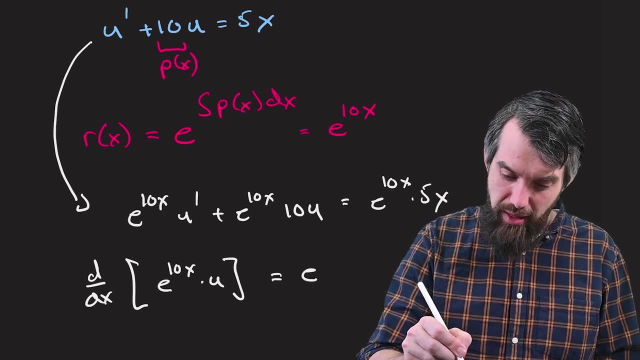 I can rewrite this left-hand side as the integral of e to the 10x, the integrating factor, and then just multiply it by u And by product rule. that's the same thing, And on the left nothing changes. so I'll just copy that down one more time. 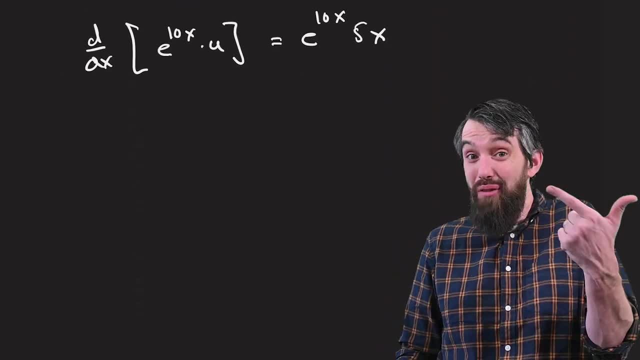 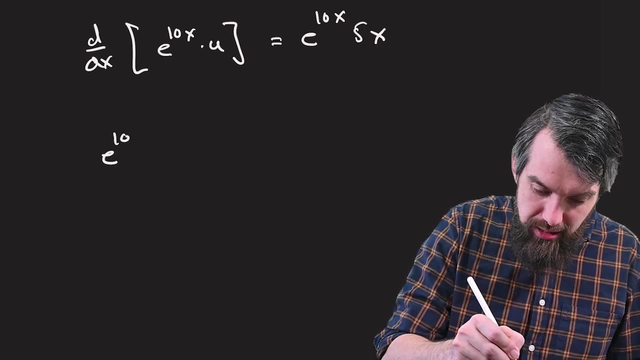 Okay, so that's the thing that we now want to do. But I can solve that differential equation. Just a derivative is equal to something, So integrate both sides. On the left, you get e to the 10x multiplied by u. 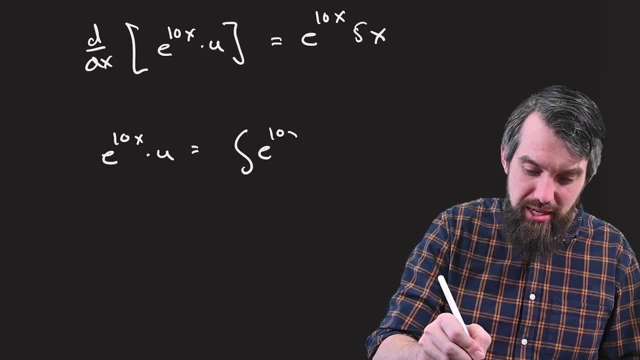 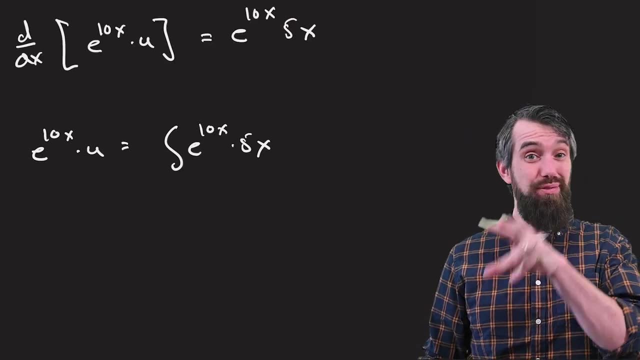 And on the right-hand side you have the integral of e to the 10x, So e to the 10x multiplied out by 5x. Now we can do this integral. It looks like e to the 10x times 5x. 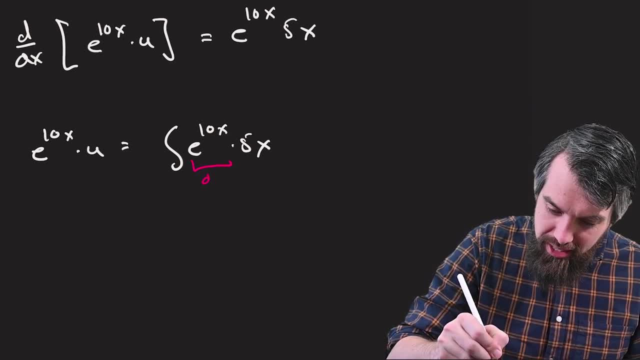 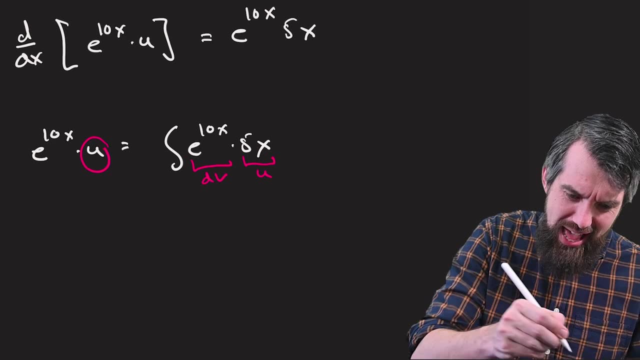 That's going to be an integration by parts, So I'll come here and do a very quick dv and u. This u and v is just the standard nomenclature for integration by parts. I'm not trying to relate it to that u at all. 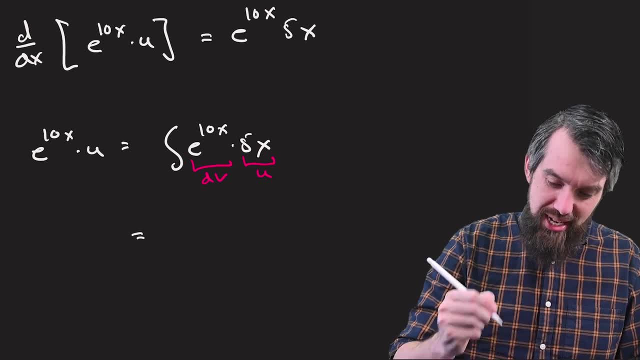 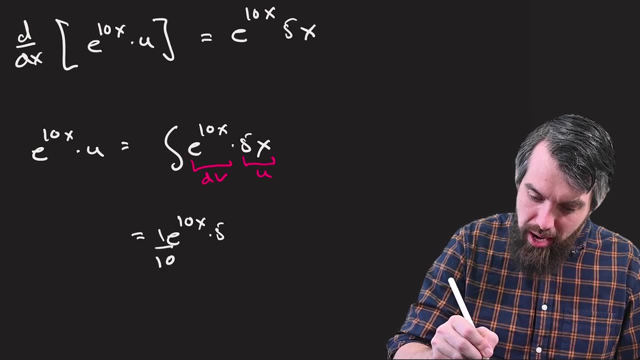 This is just a temporary thing for solving our integral here. Anyways, what is it? It integrates to u times v, so e to the 10x and then divide it out by 10.. Multiplied by 5x minus the integral of v to u. 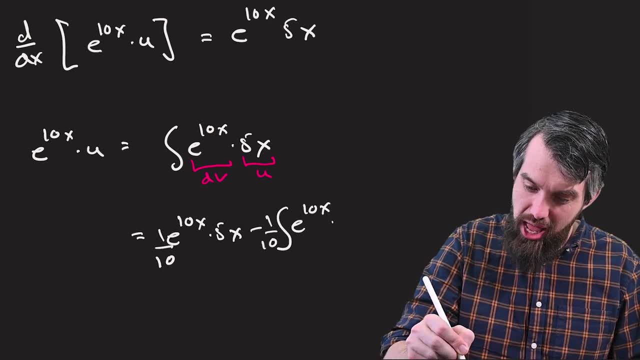 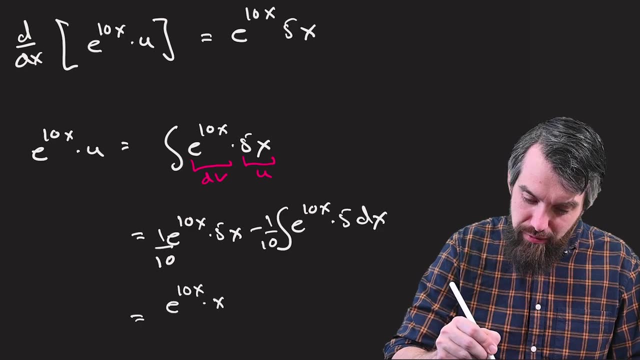 So I have 1 tenth e to the 10x times 5dx. Finally, I can come here and say this is going to be e to the 10x times x divided out by 2. And then when I integrate I get minus 1 hundredth.